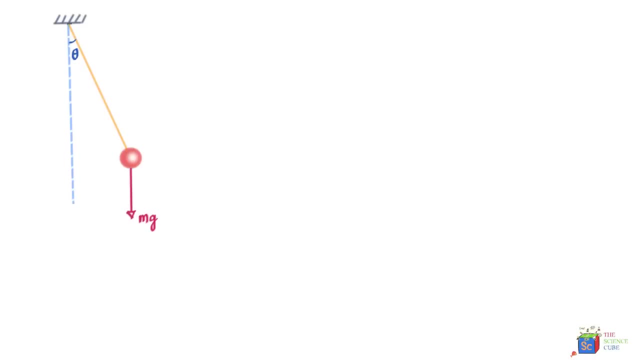 and the tension in the string that tends to pull the ball in upward direction. and let's say the length of the string is L over here. So let's go ahead and mark L and the tension T in the string. So let's say this is length L and the tension in the string is T, and you can see that the ball will. 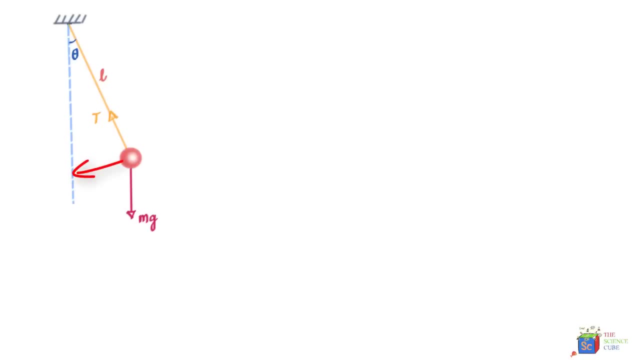 arc and oscillate, and let us label this as motion in x direction and this in y direction. So if you decompose tension T in its respective components, you have T cos theta as a vertical component, because this angle will also be theta. The horizontal component will be T sin theta. Now we know that Newton's second law of motion 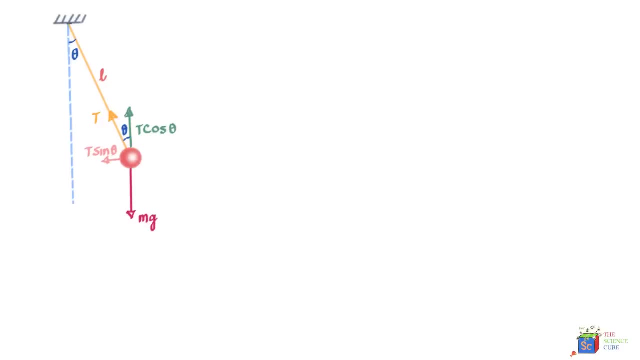 says that force on a body is equal to the product of mass and acceleration, and it's so often written as F is equal to m into a. So let's go ahead and write the force equation for x and y direction separately. So in x direction the only force we can see is T, sin theta. So we 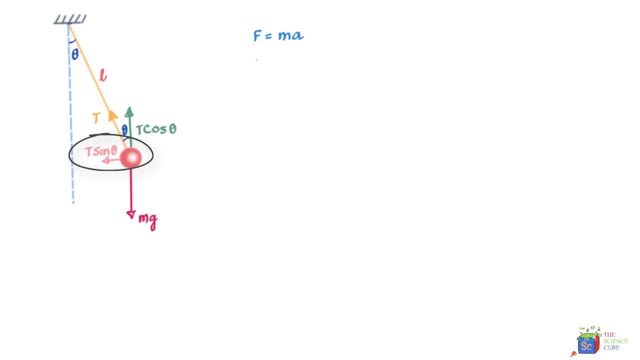 can write well, m, a is equal to, and we'll write a as a x, which essentially tells its acceleration in x direction, and this should equal to minus T, sin theta. and we've put the minus sign because it's a restoring force and it's bringing it back towards the center, towards the left, and 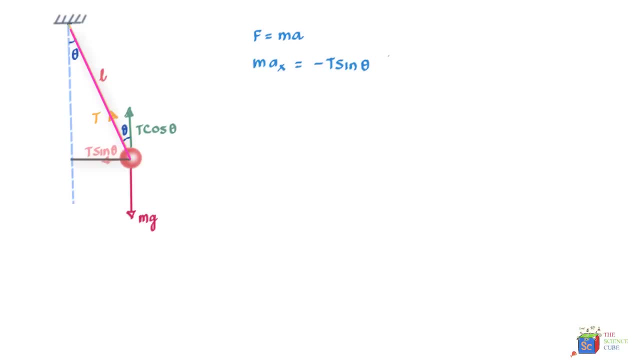 well, we also know that sin theta is nothing but x upon L, and we must qualify here that here x is equal to zero and this is actually positioned x, and if this is the case, then this distance is x and sin theta would be x upon L. So let's write this as equal to minus T into x upon L, where L is. 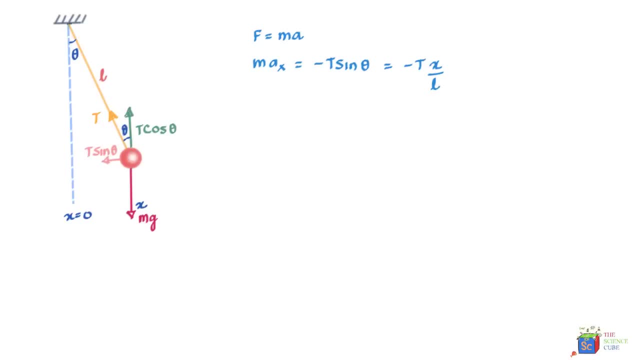 the length of the pendulum, or length of the string, and let's say this is our equation number. well, if you were to write the same equation- Newton's second law of motion- for y direction- what we'll get is m into a y, where a y is the acceleration of the ball in in the y direction. 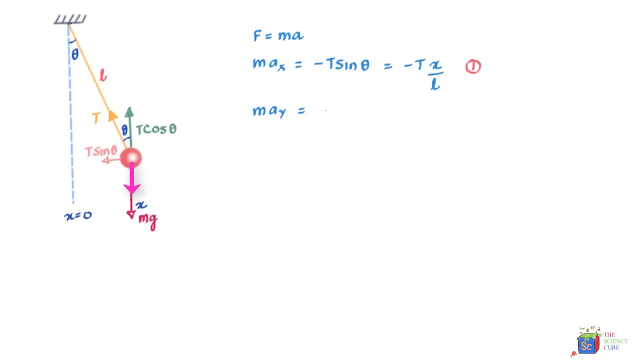 should equal to T cos theta, which is acting in the upward direction, minus mg, which is acting in the downward direction. So this is the second equation we have in the y direction. so we can say: this is in x? x direction and this is in y? y direction. So in: 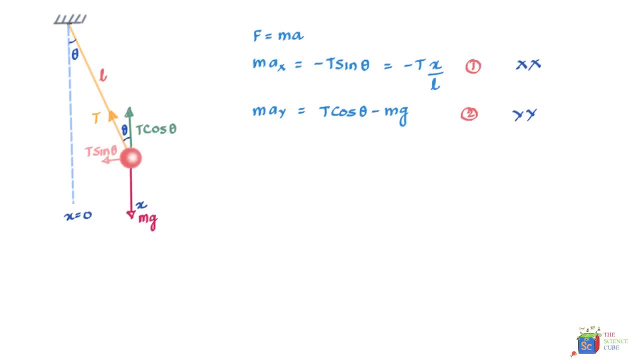 physics, we make a lot of assumptions and we'll make two assumptions over here. in fact, we'll make one assumption and the second one would be an outcome of the first assumption. So first assumption is called the small angle approximation. Well, the small angle approximation assumption is: 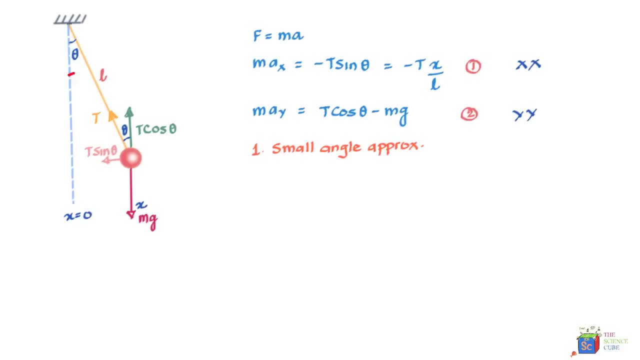 that the displacement of the pendulum will be through a small angle only, since for larger angles the pendulum will not exhibit simple harmonic motion. In fact, smaller the angle, more perfect the simple harmonic motion would be. So we'll assume that the ball does not move beyond, say, 10 degrees and, as I said, 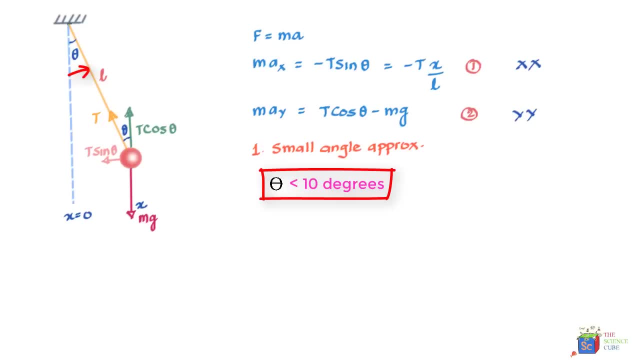 smaller the angle, the better it is. Well, if this is the case, then the cos of the angle will be close to one. and how close to one would that be? well, at five degrees, cos of 5 is 0.996, which is quite close to 1.. In fact, even at 10 degrees it is 0.985. that is cos. 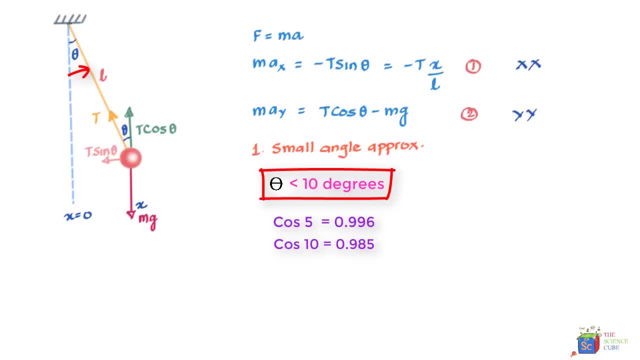 of 10 degrees is 0.985, which actually is about 1.5 percent of 1.. So still very close. So if this is the case, we can say that cos of theta, where theta is the angle of displacement and is very small- typically less than 10 degrees or even lower- cos of theta should be approximately equal. 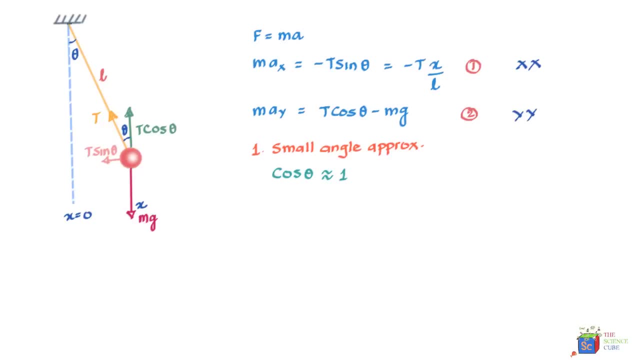 to 1.. As a consequence of this small angle assumption, what you'll find is that the acceleration of the ball in vertical direction will be very small. So if this is the arc of movement, then you can say that this is x displacement and this is y displacement, and for small angles. 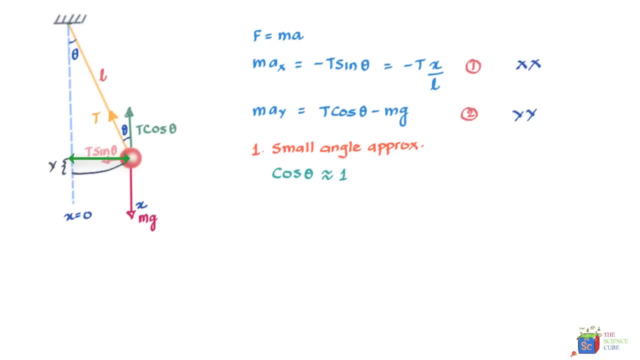 you can say that this is x displacement and this is y displacement. So if this is the arc of movement, what you'll find is- and you can go ahead and derive yourself- that y would be significantly smaller than x. and if this is the case, what you'll find is that the acceleration of the ball 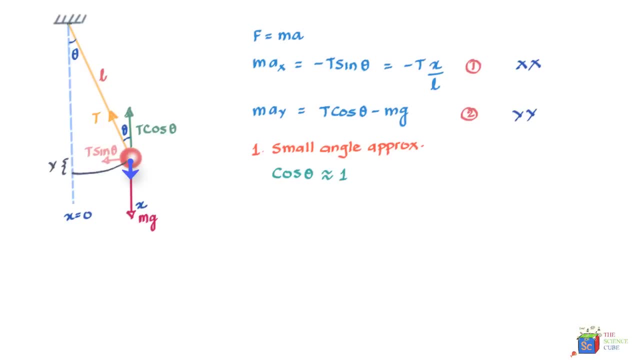 in vertical direction will be very small, and this is true since the displacement of the ball in vertical direction for low theta values is very small. In fact, at 5 degree displacement, the y displacement will be just 4.5 percent of the x displacement. So the second assumption is: 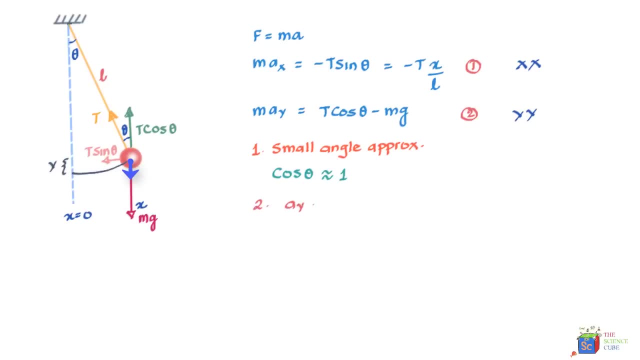 that acceleration in the y direction is approximately equal to 0. Well, if these are the two conditions, then equation 2 becomes this: So let's go ahead and put on the left hand side, a y is equal to 0 or it's approximately equal to 0. So we'll take it as 0 here. So the left hand side. 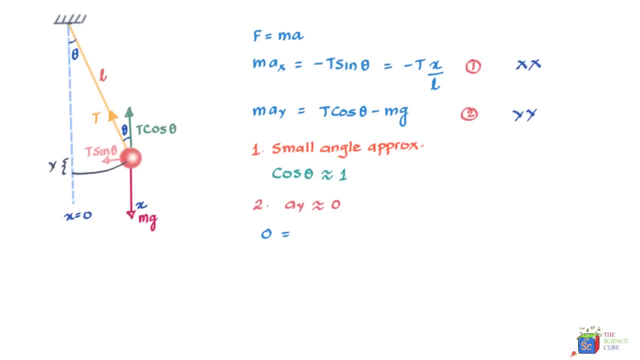 becomes 0, and this should equal to t cos theta, and we assume that cos theta is very close to 1.. So the expression t cos theta becomes t only, and you have minus mg over here, and what you get is therefore: t is equal to mg. Well, if we substitute the value of t as mg in equation 1, what you get 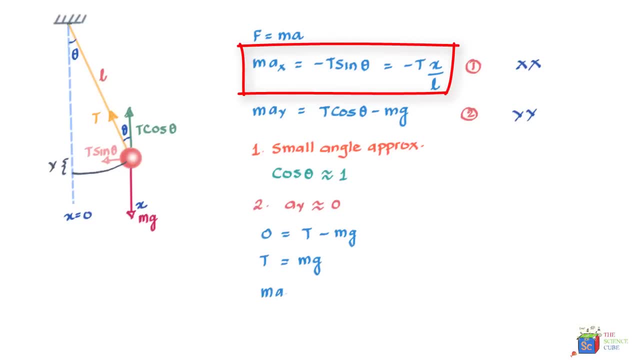 is m into ax or acceleration x direction should equal to minus mg. we've substituted the value of t as mg into x upon l and what we can see is that m is cancelling off from both sides and what we're getting is ax or acceleration in x direction is equal to minus g. 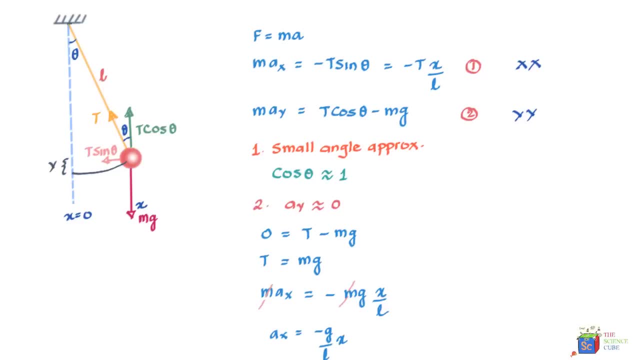 upon l into x, which is nothing but the equation of simple harmonic motion. and it is so because, if you recall from the earlier lessons, the equation of simple harmonic motion is the equation of condition for simple harmonic motion is that displacement and acceleration should be opposite in directions at all times and the two variables need to be connected by a certain 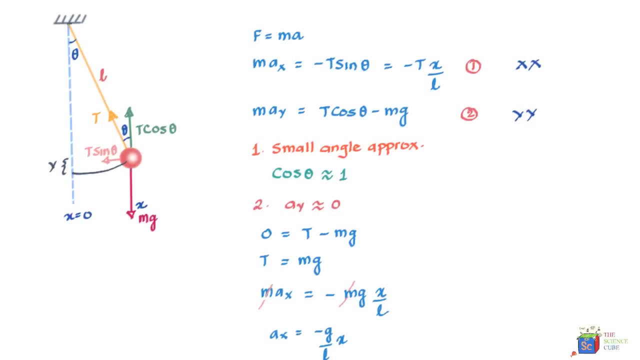 constant which was, if you recall, k upon m in case of springs. So you can see that this equation is also satisfying conditions of simple harmonic motion, and here k upon m has been substituted by g upon l. We know that ax is also equal to minus omega square x, where omega is a angular frequency, which therefore,